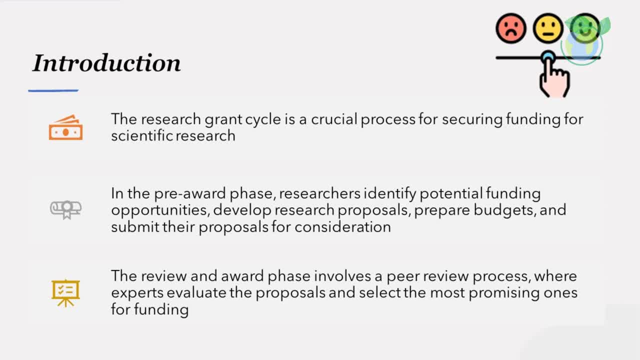 phase. In the pre-award phase, researchers identify potential funding opportunities, develop research proposals, prepare budgets and submit their proposals for consideration. The review and award phase involves a peer review process where experts evaluate the proposals and select the most promising ones for funding In the post-award phase. 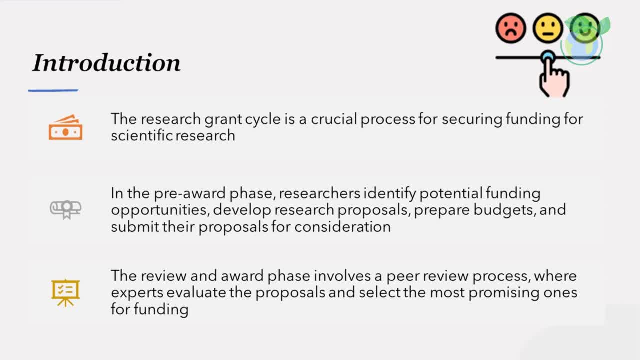 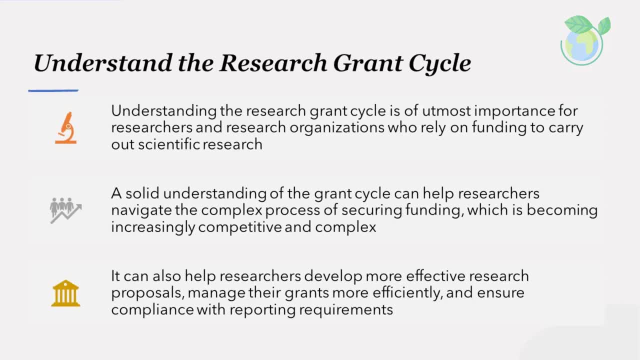 grant recipients must manage and administer the award, including reporting requirements, budget management and project monitoring and evaluation. Understand the research grant cycle. Understanding the research grant cycle is of utmost importance for researchers and research organizations who rely on funding to carry out scientific research. 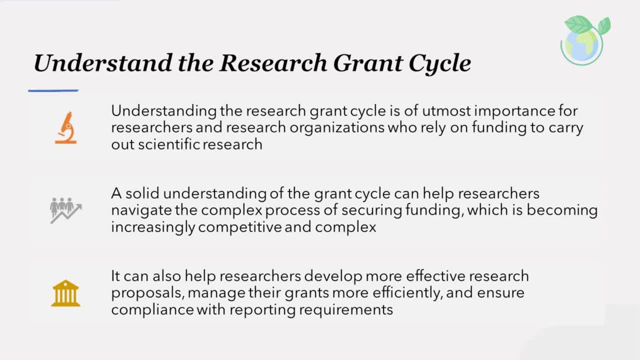 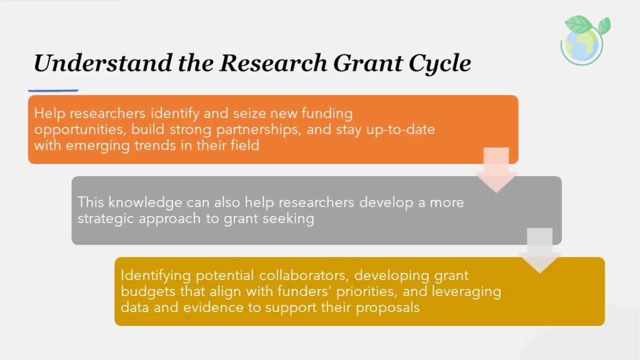 A solid understanding of the grant cycle can help researchers navigate the complex process of securing funding, which is becoming increasingly competitive and complex. It can also help researchers develop more effective research proposals, manage their grants more efficiently and ensure compliance with reporting requirements. Understand the research grant cycle. Moreover, understanding the research grant cycle can help. 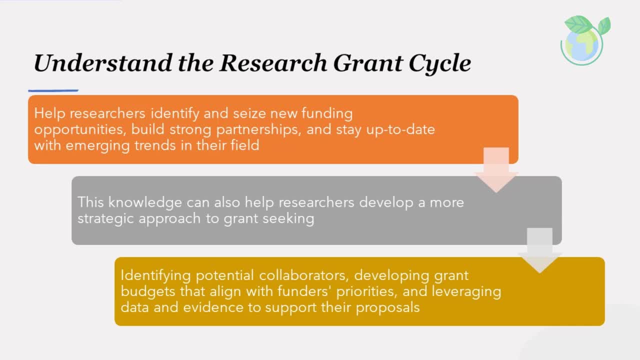 researchers identify and seize new funding opportunities, build strong partnerships and stay up-to-date with emerging trends in their field. This knowledge can also help researchers develop a more strategic approach to grant seeking, including identifying potential collaborators, developing grant budgets that align with funders' priorities and leveraging data and evidence to support their proposals. 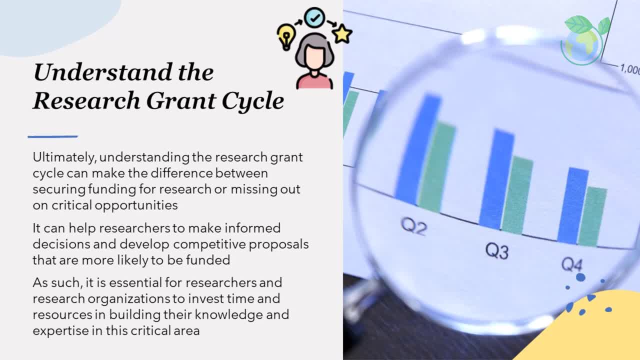 Ultimately, understanding the research grant cycle can make the difference between securing funding for research or missing out on critical opportunities. It can help researchers to make informed decisions and develop competitive proposals that are more likely to be funded. It can also help researchers to make informed decisions and develop competitive proposals that are more likely to be funded. 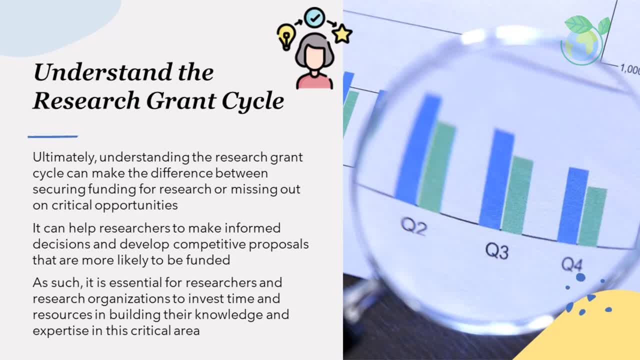 It can also help researchers to make informed decisions and develop competitive proposals that are more likely to be funded. It can also help researchers to make informed decisions and develop competitive proposals that are more likely to be funded. As such, it is essential for researchers and research organizations. 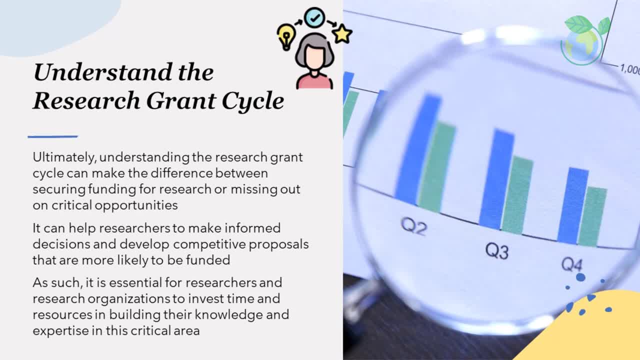 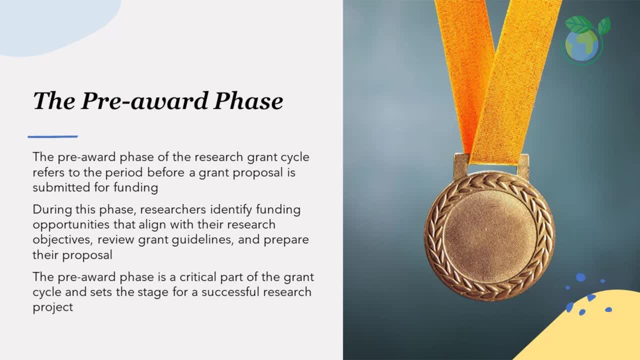 to invest time and resources in building their knowledge and expertise in this critical area. The Pre-Award Phase. The pre-award phase of the research grant cycle refers to the period before a grant proposal is submitted for funding. During this phase, researchers identify funding opportunities. 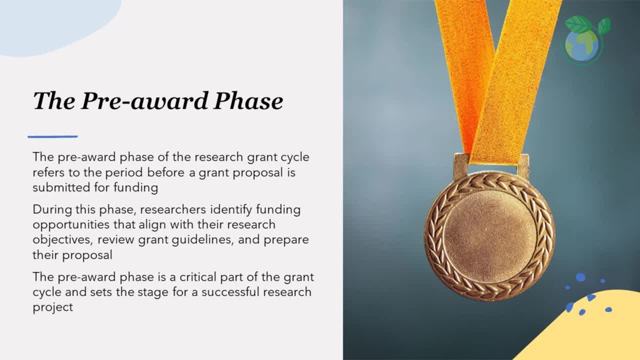 that align with their research objectives, review grant guidelines and understand the potential role guidelines and prepare their proposal. This may include tasks such as identifying potential collaborators, developing a budget and creating a detailed project plan. Additionally, researchers may need to secure institutional approvals, such as obtaining 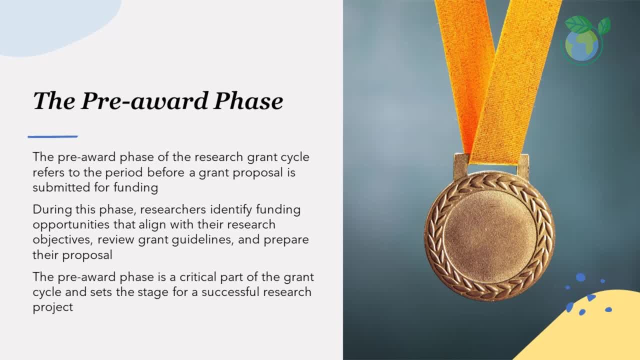 signatures from department heads or submitting required documentation to the institution's grants office. The pre-award phase is a critical part of the grant cycle and sets the stage for a successful research project. Adequate time and attention to detail during this phase can increase the likelihood of 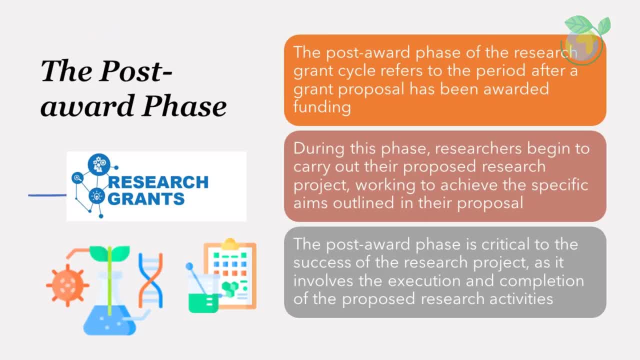 a successful grant proposal submission. The post-award phase. The post-award phase of the research grant cycle refers to the period after a grant proposal has been awarded funding. During this phase, researchers begin to carry out their proposed research project, working to achieve the specific aims outlined in their proposal. 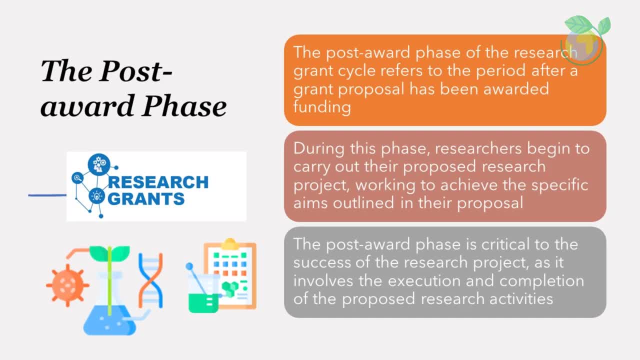 This may include activities such as conducting experiments, collecting and analyzing data and disseminating research findings. Additionally, researchers must adhere to any reporting and compliance requirements specified by the funding agency. This may include submitting regular progress reports or final reports summarizing project outcomes, as well as complying with any regulatory requirements related to the use of human or 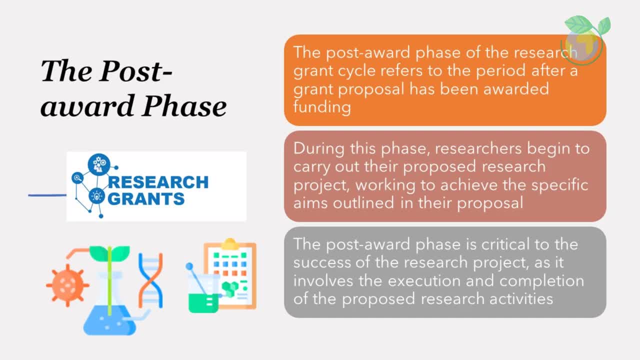 animal subjects. The post-award phase. The post-award phase. The post-award phase is critical to the success of the research project, as it involves the execution and completion of the proposed research activities. Proper management of the project during this phase can help ensure that the research objectives. 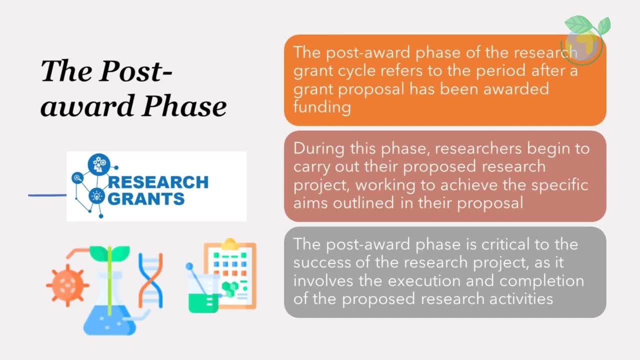 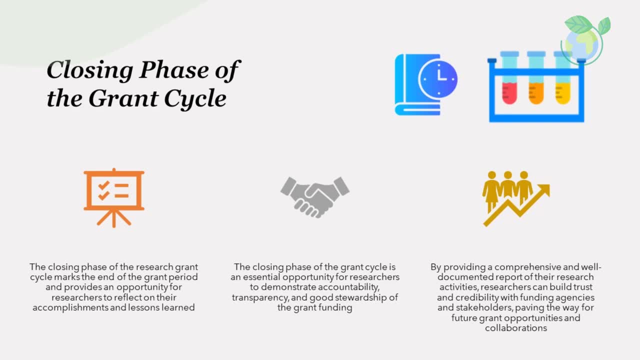 are achieved and that the grant funding is used effectively and efficiently. Closing phase of the grant cycle. The closing phase of the research grant cycle marks the end of the grant period and provides an opportunity for research To reflect on their accomplishments and lessons learned during this phase. researchers typically 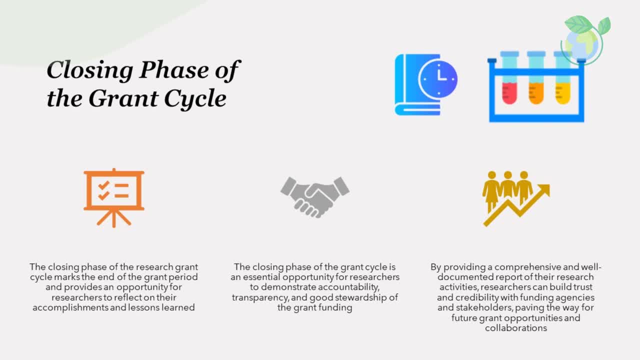 submit final reports and any required deliverables to the funding agency. This may include summaries of research findings, dissemination activities and any impact the research had on the broader scientific community. Additionally, researchers may use this time to evaluate the project's success identify. 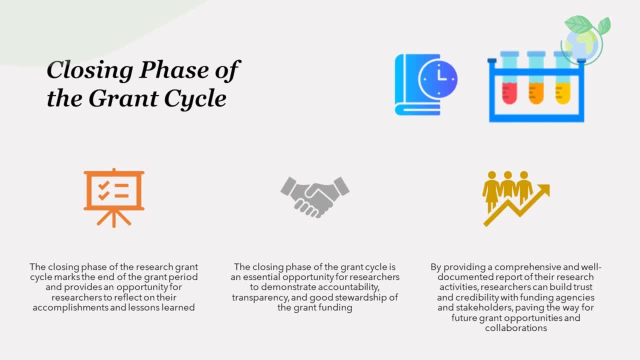 any challenges or unexpected outcomes. The closing phase of the grant cycle is an essential opportunity for researchers to demonstrate accountability, transparency and good stewardship of the grant funding. By providing a comprehensive and well-documented report of their research activities, researchers can build trust and credibility with funding agencies and stakeholders, paving the way. 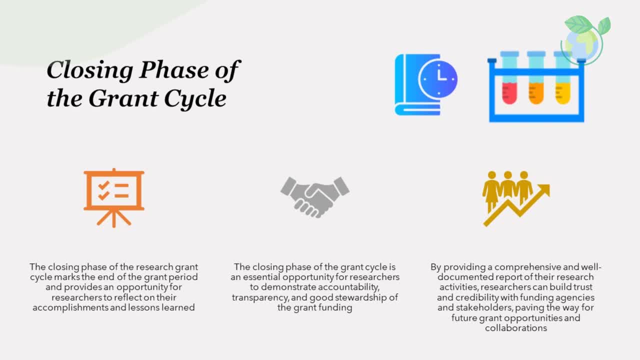 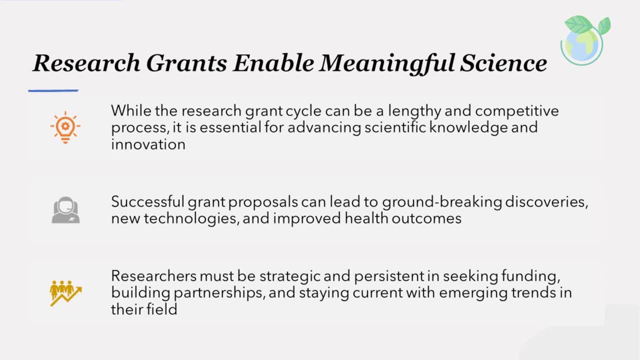 for future grant opportunities and collaborations. Research activities- Research activities- Research grants enable meaningful science. While the research grant cycle can be a lengthy and competitive process, it is essential for advancing scientific knowledge and innovation. Successful grant proposals can lead to groundbreaking discoveries, new technologies and improved 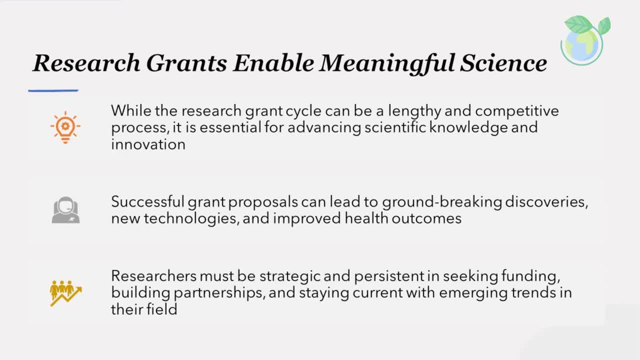 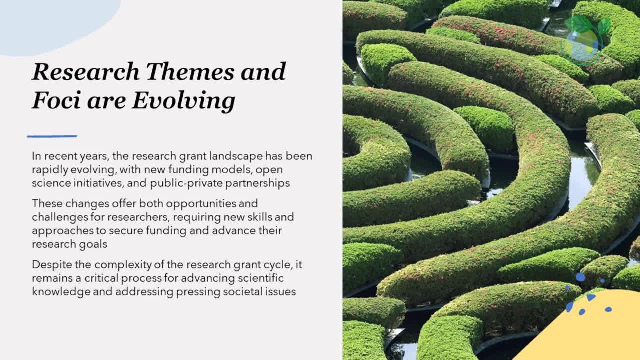 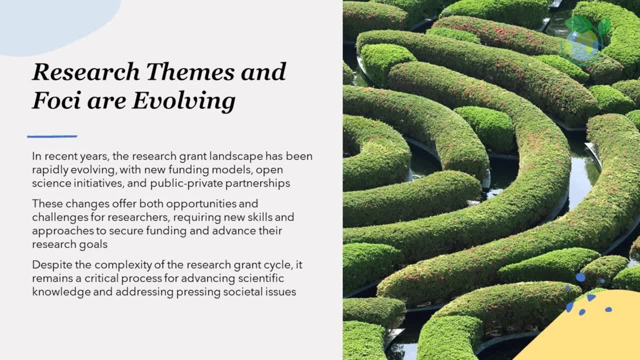 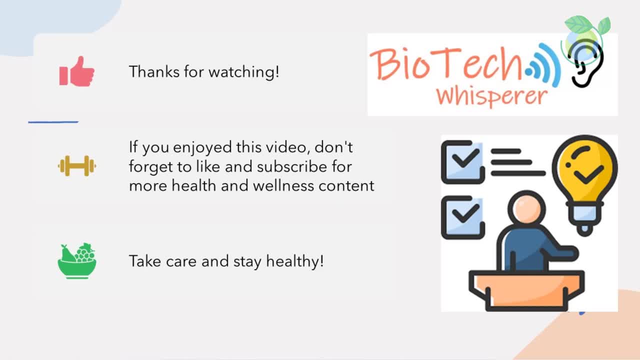 If you're enjoying the content you're seeing here, be sure to give us a like and hit that subscribe button to stay up to date on all our latest videos. Liking our videos not only shows us that you appreciate the content we're creating, but 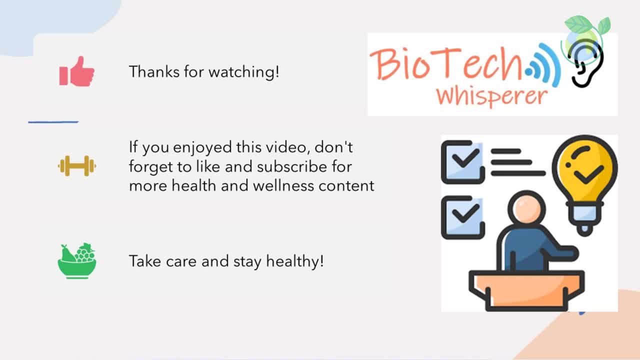 it also helps our videos reach a wider audience. Subscribing to our channel means you'll never miss a video and you'll be the first to know when we upload something new. Plus, it's completely free. So what are you waiting for?